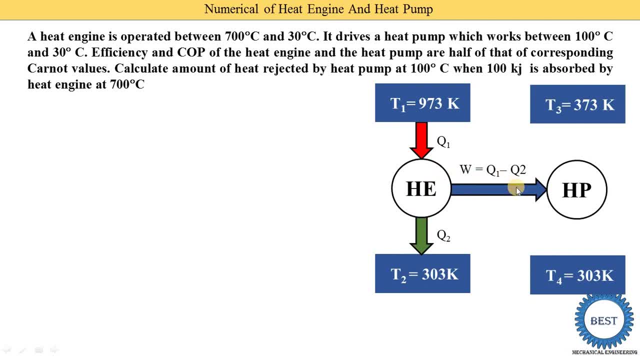 This heat pump is runs by using the work done produced by the heat engine and this heat. the pump is worked between the temperature of 100 degree, means 373 kelvins, and the sink temperatures for the heat pump is the 30 degree centigrade means 303 kelvins. heat pump is absorbed the q4. 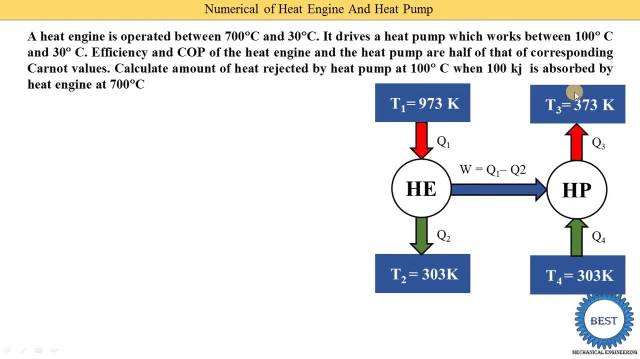 quantity of the heat energy from the sink and supplied it to the source. that is a q3 quantity and under the data is given: efficiency and cop of the heat engine and the heat pump are half or that of the corresponding Carnot values. so here we mention this data. okay, first we may write down. 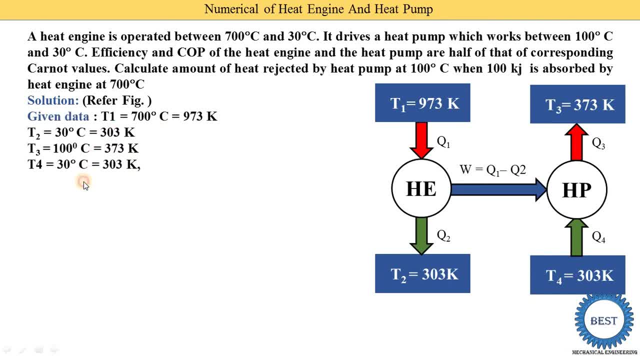 this t1, t2, t3 and t4. then after actual efficiency is given, 50 percent of the maximum efficiency means here half of the corresponding Carnot value is given. so first we need to find out the Carnot efficiency. from the Carnot efficiency we find out the actual efficiency. same data is given for the 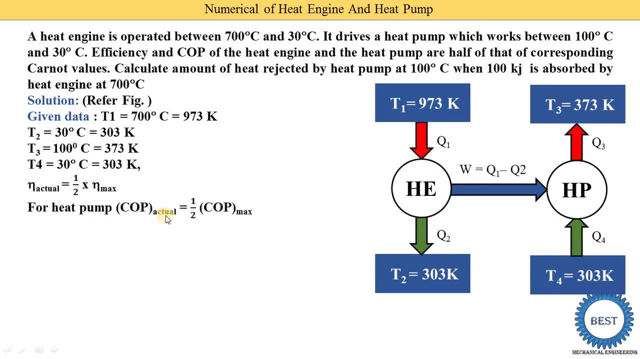 cop of the heat pump. so for the heat pump, cop actual is one half of the cop maximum, means the actual cop is 50 percent of the maximum cop. we need to calculate amount of heat rejected by a heat pump at 100 degree centigrade. so here you see, this is. 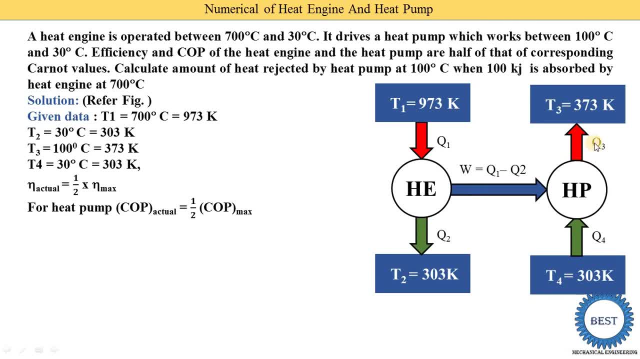 the 100 degree centigrade. okay. so here, amount of heat rejected is the q3. so we need to find out the q3. okay, when 100 kilojoule is absorbed by a heat engine at 700 degree centigrade means q1 is given. 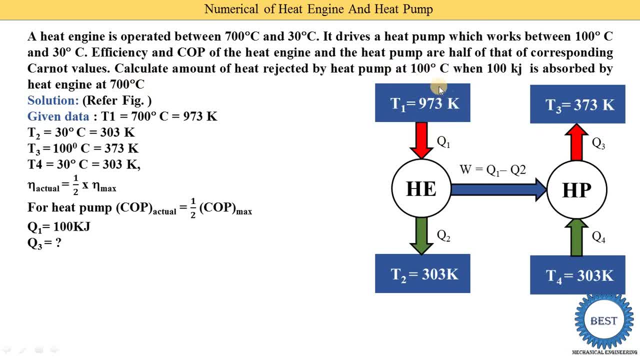 okay, so here that is the amount of heat rejected by a heat pump at 100 degree centigrade. so here that is the 700 degree centigrade for the heat engine, and here the heat engine is absorbed. the 100 kilojoule means this is the q1 is given. so here we mentioned q1 is equal to 100 kilojoules. 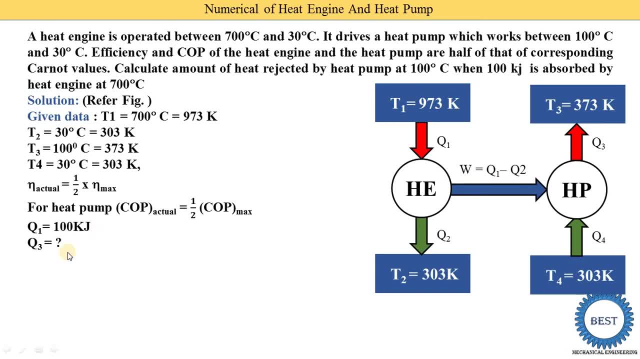 and we need to calculate the q3. so first we are find out the all the unknown parameters of the heat engine, because it is the basic things, okay, so here t1 and t2 is given, q1 is given. so first we find out the efficiency of the heat engine, then we find out the q2 and w, then, after we are, find out. 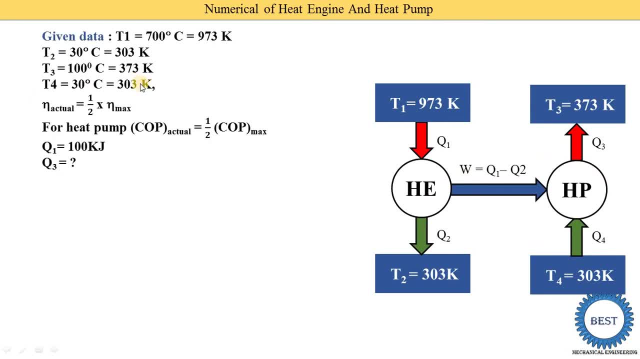 all parameters for the heat pump. so here we mentions the what amount of the given data. so what is the given data is written that we take again here, okay. so first we solve the problem of the heat engine. for the heat engine, first we find out the Carnot. efficiency means the. 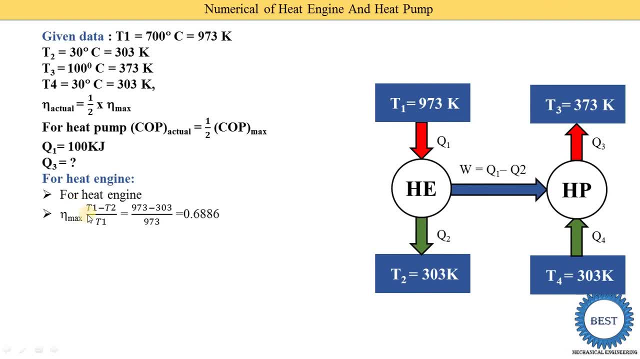 maximum efficiency. so this Carnot efficiency is find out from the temperatures. it is the t1 minus t2 upon t1 that we already derived these equations for the Carnot efficiency and in efficiency and uop equations we need to put all the temperatures in the Kelvin, okay. so here we putting t1, that is. 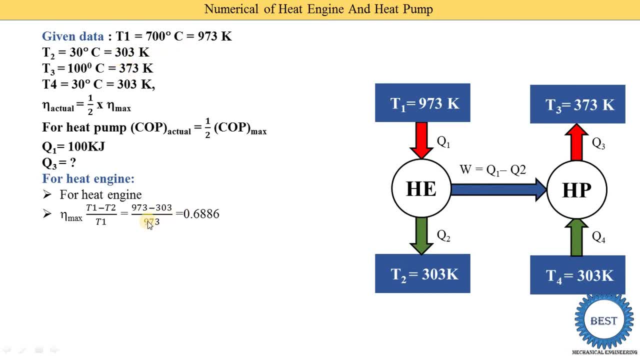 a 973. t2 is given, 303 divided by t1, that is a 973, and we get this answer: that is 0.6886. efficiency and this is the maximum efficiency. okay, and related to efficiency, the actual efficiency is given. it is a 1 by 2 of the maximum efficiency. so actual efficiency is 1 by 2 of the maximum. 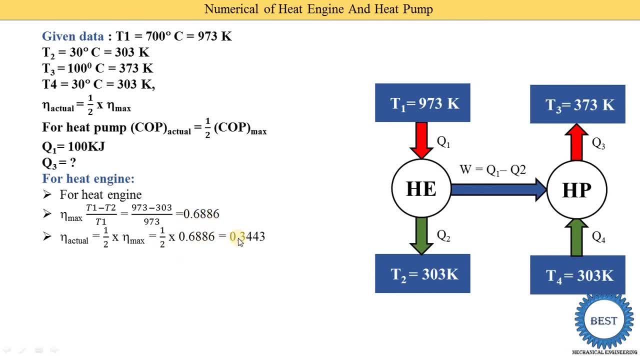 efficiency. so maximum efficiency is 0.6886, so actual efficiency is 0.3443 and we know that is the actual efficiency equations. that is the output upon input. okay, so what is the output for the heat engine? output for the heat engine is the work done. 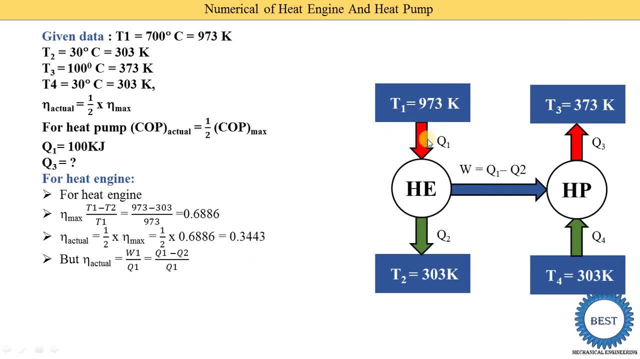 okay, that is the w1. and what is the input? input for the heat engine is the q1. okay, so we return. that is a actual efficiency is equal to w1 upon q1, and w1 is also written as the q1 minus q2. so here we return. it is a q1 minus q2 divided by q1s, so we know the maximum. 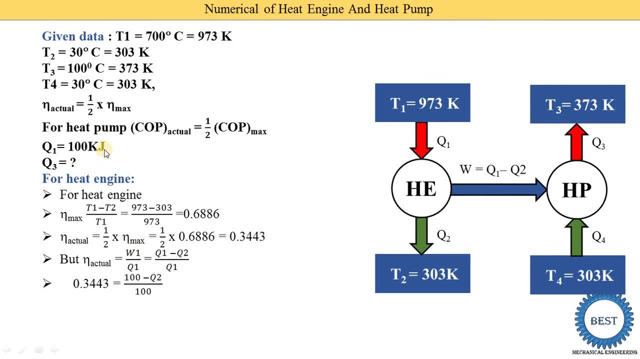 sorry, actual efficiency: it is a 0.3443. q1 is already given. there is a 100 kilojoule, so we putting q1 is equal to 100 kilojoules, okay, and by using these calculators we are find out this q2. so 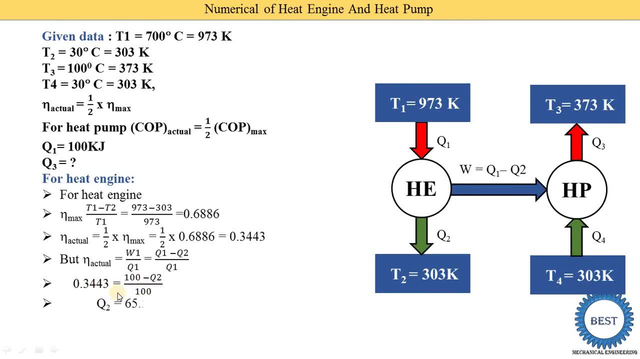 this 100 is supply on the left sides. then further we simplify, then we get this answer: q2 is equal to 65 point 57 kilojoule, so work produced by the engine is: w is equal to q1 minus q2, so it is the 100. 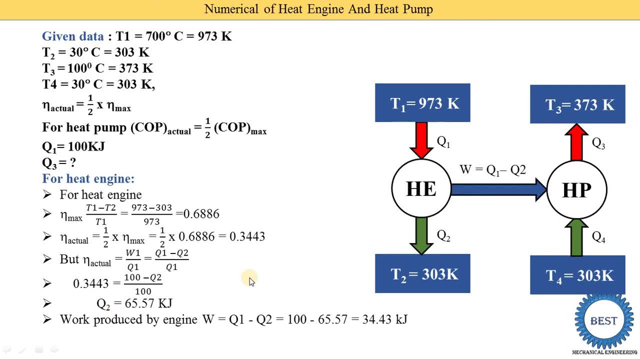 minus q2. okay, so here we find out q2. so here only remaining parameter is the work done. so work done is equal to q1 minus q2. so q1 is given 100 kilojoule. we find out the q2, so q2 is 65.57. 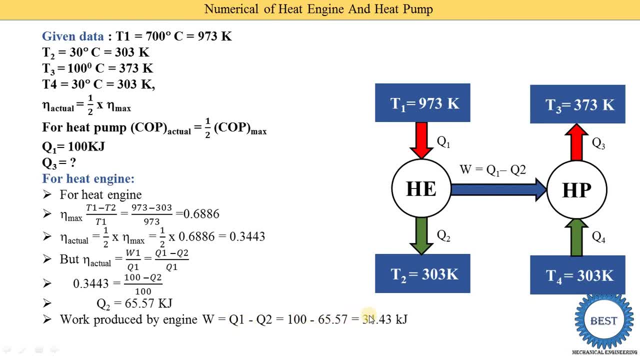 then we get the answer of the work done. so answer of the work done is 34.43. okay, so here we are, find out all the parameters, that is, the q2 and the work done and the efficiency. now we need to move to the heat pump. okay, so in a data it is given that the work produced by the heat engine 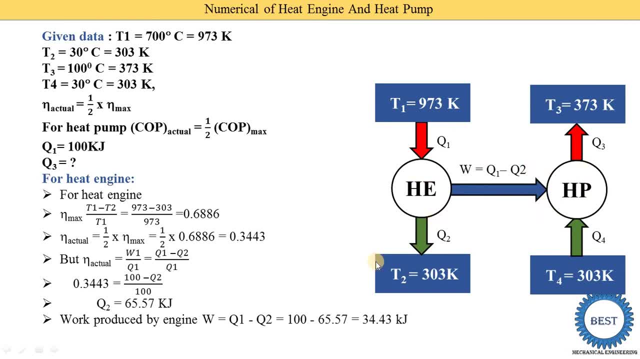 is completely supplied to the heat pump means here: work supplied to the heat pump is equal to work produced by the engine. so work done. supply to the heat pump is also 3.443 kilojoules, and now we are find out the q3. okay, now, before moving that, i request to like the video and subscribe my channels for watching the more video related videos. 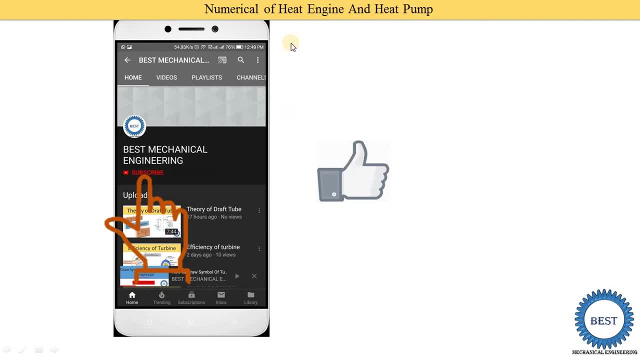 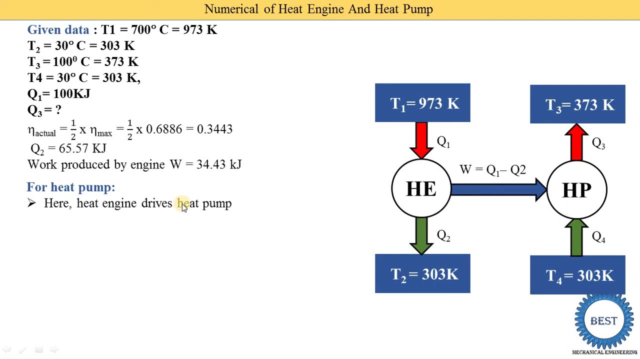 to engineering thermodynamics, another subject of mechanical engineering. for engineering thermodynamics, whereas link is provide in descriptions and card for other subject, i request to visit the playlist. now we solve the heat pump, so in a heat pump we need to find out the cop. okay, so suppose. 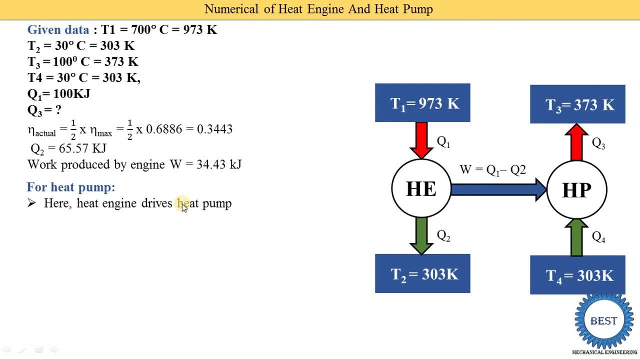 any combined numerical is asked. so first you need to find out the efficiency and the cop- suppose heat engine is that- and we find out efficiency, heat pump given and we need to find out the cop. okay, this is the first basic step for the numericals of heat engine and heat pump. so for a heat pump the heat engine drives, the heat pump means. 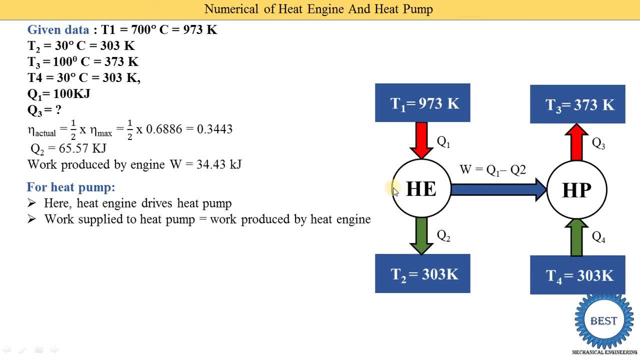 work supplied to the heat pump is equal to the work produced by a heat engine. so work produced by heat engine is 34.43. that we already find out, okay. so what is the equations for the work supplied to the heat pump? it is the q3 minus q4, okay, or we also written: it is a w, that is a 34.43. 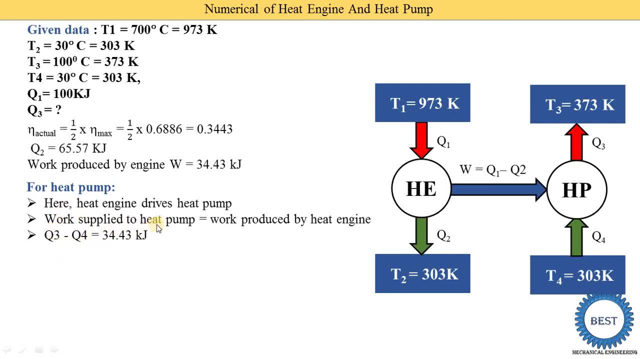 kilojoules, so how we are able to return this equation. the work supply to the heat pump is q3 minus q4. so in a heat pump- you see that is a two input, is there? okay, one is this work done and one is the q4. so this work done, w plus q4 is equal to q3. okay, so work done is equal to q3 minus q4. 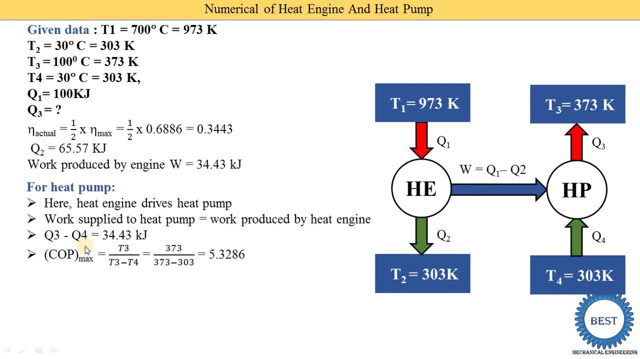 is written. now we find out the maximum cop. so here the heat pump is there. okay, so higher temperature is coming in upper part. okay, that is a t3 is higher temperature in t3 and t4. so here t3 divided by t3 minus t4. suppose here the refrigerator is given instance of this heat pump, then the 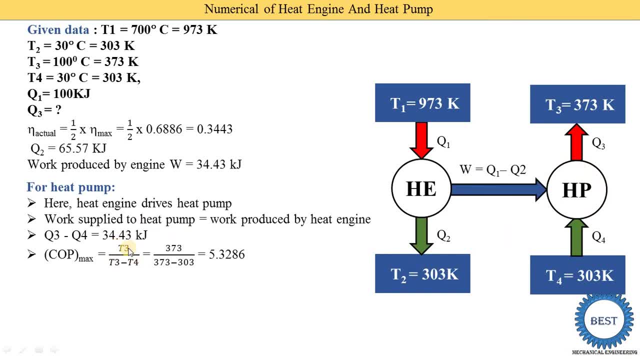 equation is changed. that is a t4 divided by t3 minus t4. t3 is given 373 kelvin, t4 is given 303 kelvin. so we putting this value of t3 and t4 in here equation and we find out the maximum cop. it is 5.3286. then we find out the actual cop. so actual. 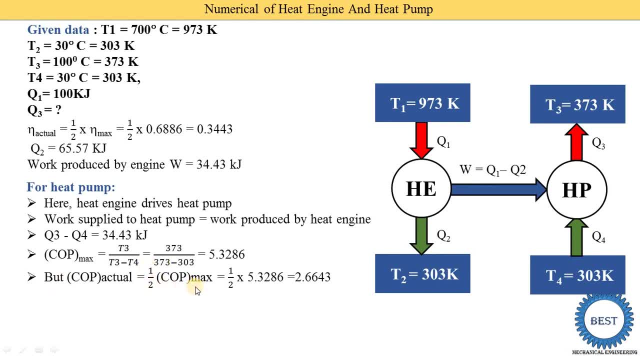 cop is 1 by 2 to the maximum cop. okay, so here the it is given in a given data. okay, so maximum cop is the 5.3286, so it is divided by 2. then we get the answer. actual cop is the two point double six. 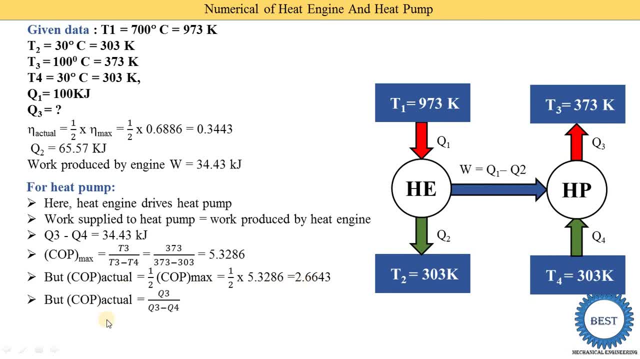 four three. so we know the equations of the actual cop, that is, the output upon input. okay, what is the output? output of the heat engine is the q3. okay, means output. heat energy is the near to the highest temperature, so here the highest template, because heat pump is used for the heating purpose. okay, so it is the q3 divided by work done. 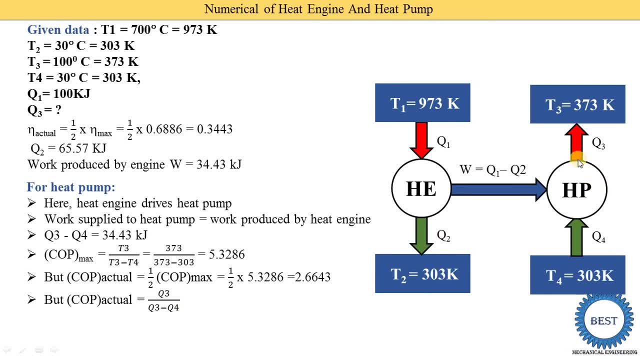 and work done is equal to q3 minus q4. suppose here refrigerator is given, then here we mentioned the q4, because refrigerator is used for the cooling purpose, so lower temperature heat interaction is considered. so here q4 is coming divided by q3 minus q4. so if a, that is a refrigerator is there. 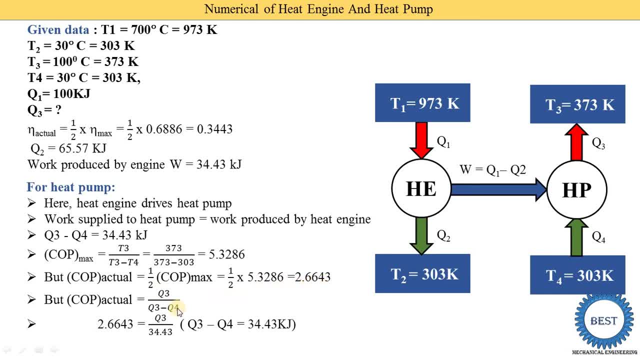 so here, actual cop, that we know that is a two point, double, six, four, three divided by q3. so we need to find out the q3 and the q3 minus q4. that is given. that is a work done. okay, that is a 34.43, so we are able to find out q3. so q3 is equal to 91.73 kilojoule heat rejected. 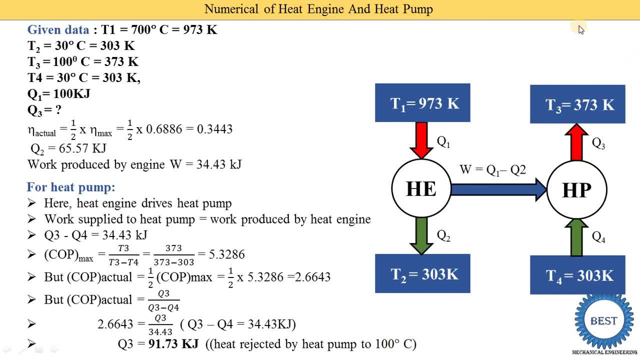 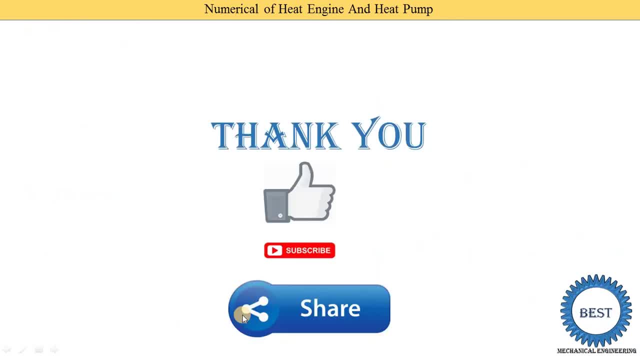 by heat pump at 100 degree centigrade. so here the t3 is the 100 degree centigrade. okay, so that is. the heat rejected by the heat pump is 91.73 kilojoules. so thank you for watching this video. if you learned something, then like the video. subscribe. my channels and don't forget to share with your friends.